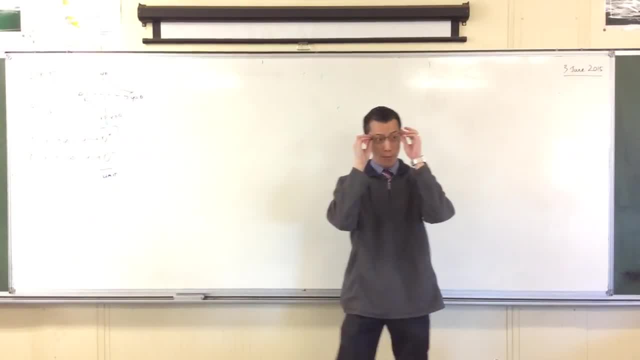 A way you can think about it is like this: If this is the analogy I gave before, If you've got a car right and you want to see as far as, as fast as it can go- right, So you're sitting in the driver's seat- you slam down the pedal, okay. 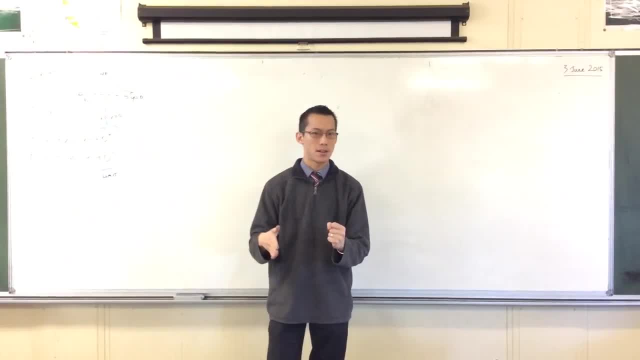 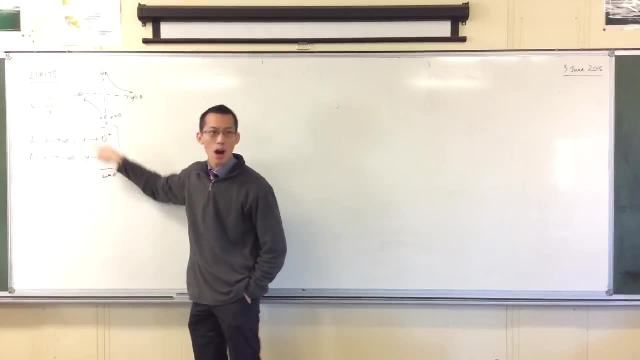 And off it goes. okay, And it's going to get faster and faster and faster, Assuming you don't brake, you don't take your foot off. okay, It's going to approach. it's going to approach some kind of speed, right? 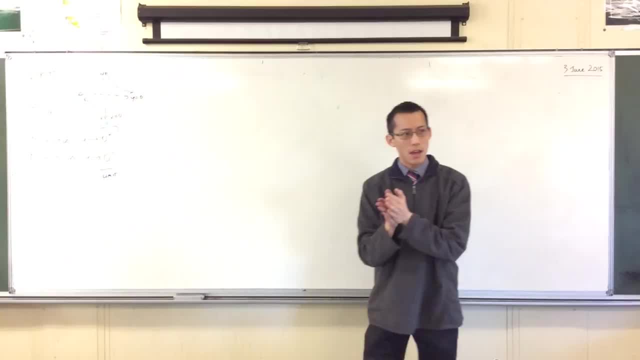 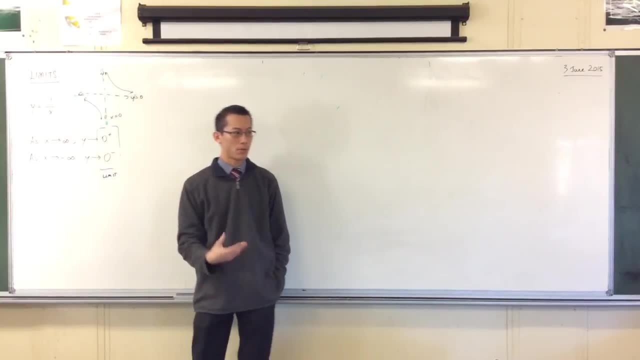 Whatever that number is going to be. Now, the flip side of saying I approach something, I approach something is to say that's my limit, That's as far as I can go. Suppose the top speed of my car is 250 kilometres per hour. okay, 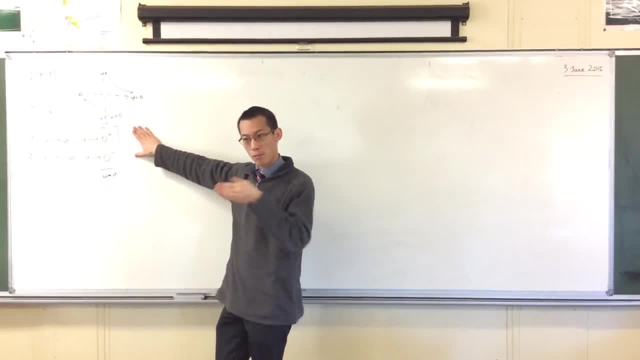 I'm going to approach that speed right. I'm going to approach, I'm going to get faster and faster and faster and faster. But from the other angle I can say that's as far as I'm ever going to go. 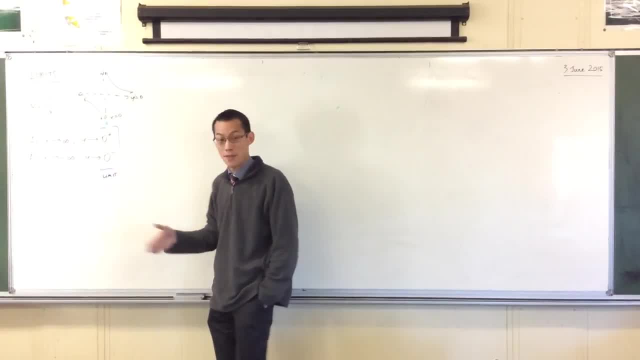 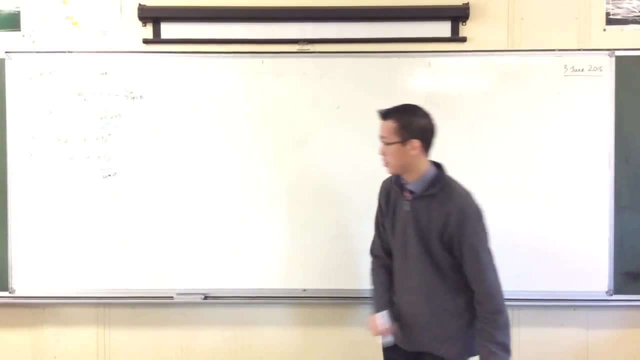 That's my limit. I will go that far and no further, okay. Or I won't even quite get there, right. That's the limit of this as it's behaving. So here's how we write this new notation, okay. 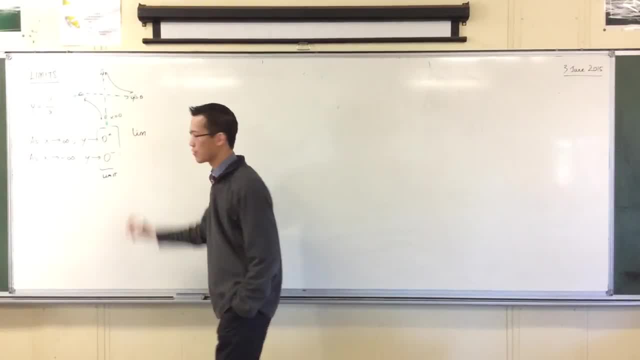 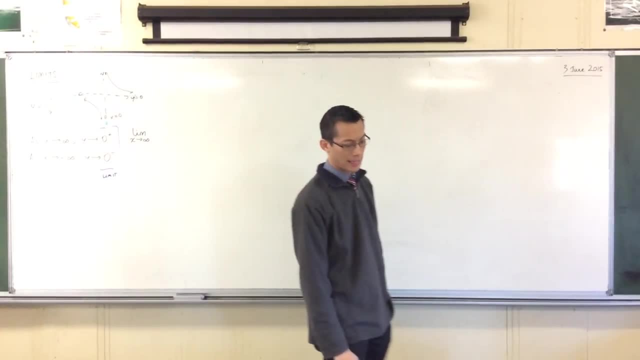 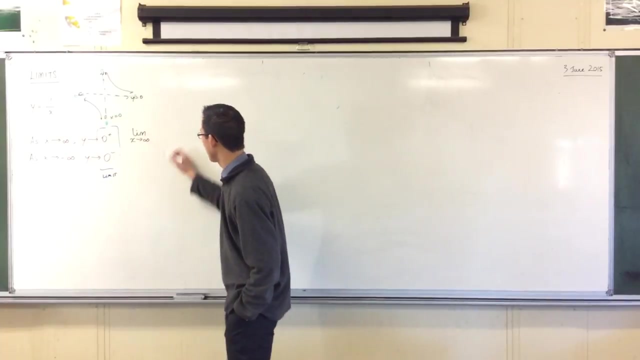 This first line, I would say the limit right Lim, short for limit As x approaches infinity. I write this underneath, Kind of like a subscript, but like it's literally underneath: Of 1 over x, right Of 1 over x. 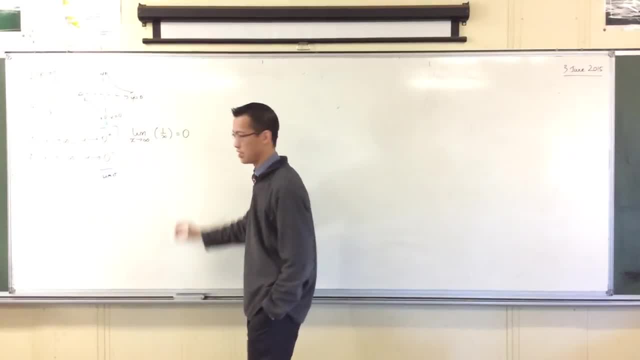 It's actually going somewhere. Namely, it's going to 0.. Okay, It's going to 0, and it's going there from above. Okay, In exactly the same way, the limit as x approaches negative infinity of the same thing: 1 over x. 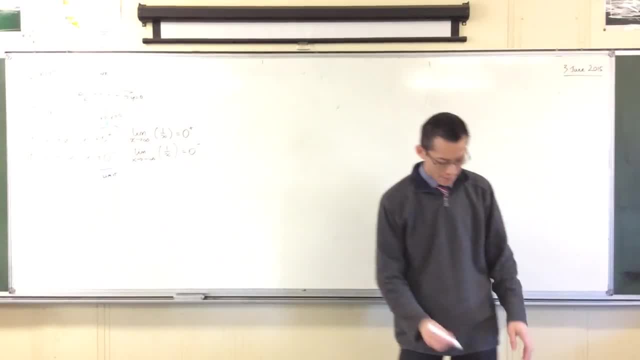 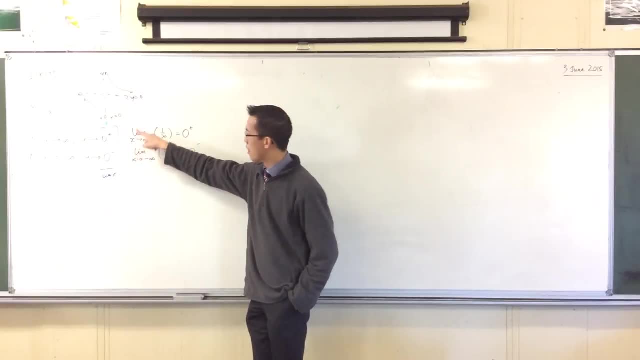 is still going to be 0, but it's from below. Okay, So I read this. Let me say this again: It's a little bit like logs with this funny way of actually saying the phrase. I read this as the limit, as x approaches infinity, of 1 over x. 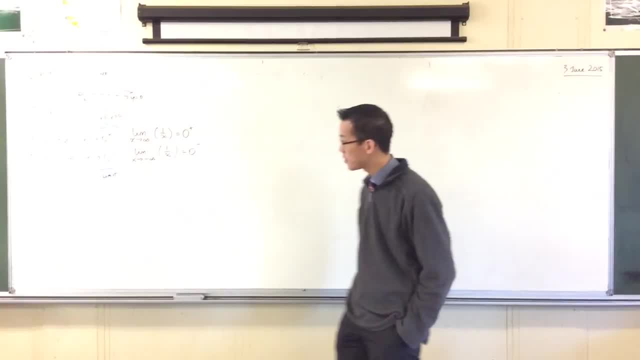 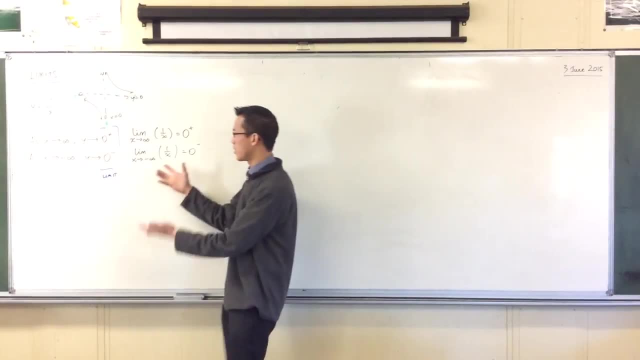 Is 0 from above The limit as x approaches infinity: 1 over x is 0 from above. Okay, Now, I'm introducing this because asymptotes are the first place where we get. we want to understand this idea of getting closer and closer and closer to something. 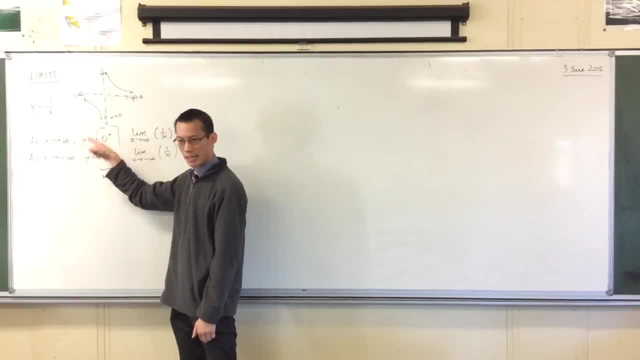 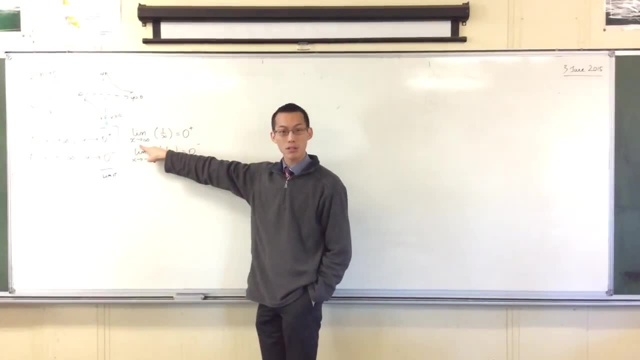 but not getting there. So all you can say- you can't say it equals in this context, right, You can only say it gets closer and closer and closer, Okay. But here I'm saying: okay, the thing that I'm getting closer and closer to is 0. 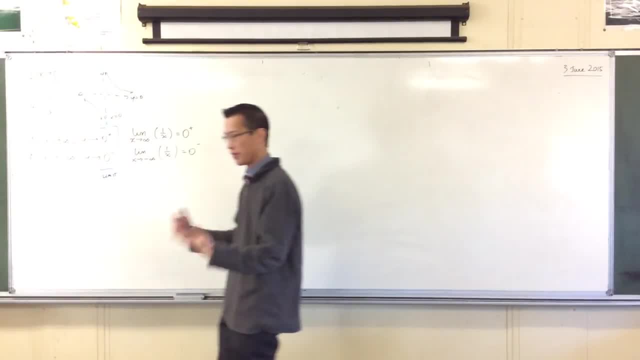 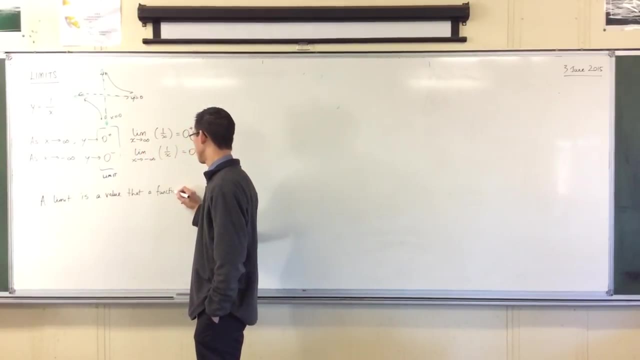 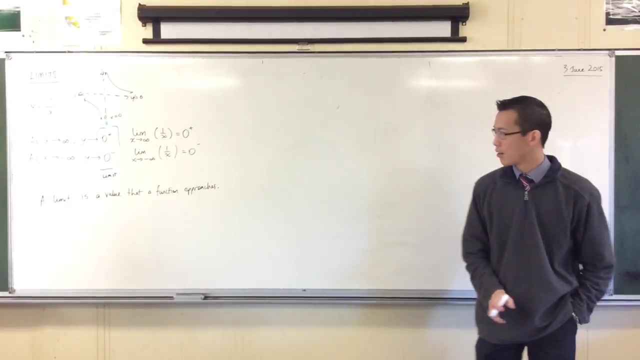 So here's my first sort of casual definition of a limit. Okay, You can put a big box around this. Okay, A limit is a value that a function approaches. Okay, That's all you need to understand. I think, Right. 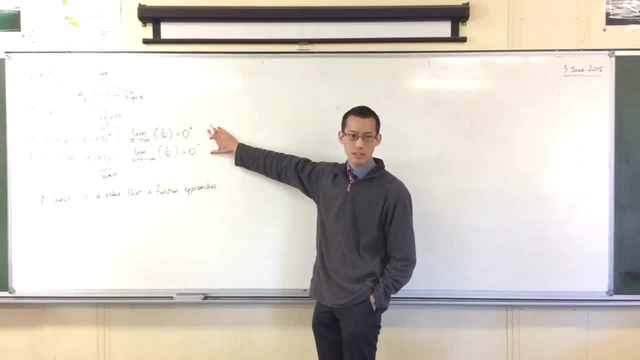 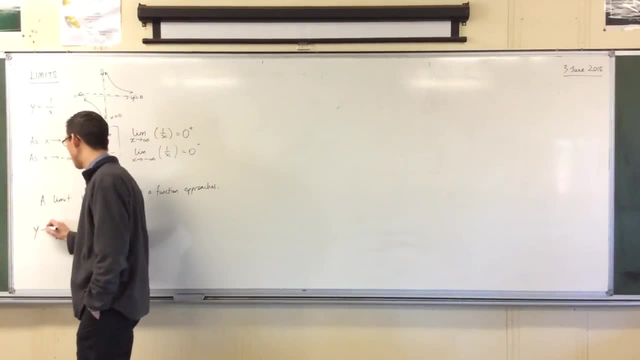 Like I'm getting closer and closer and closer to there. In these cases, I don't actually get there, But, as you'll see, there are some cases where you can just go there, Okay, For instance, let's think about a trivially simple example. 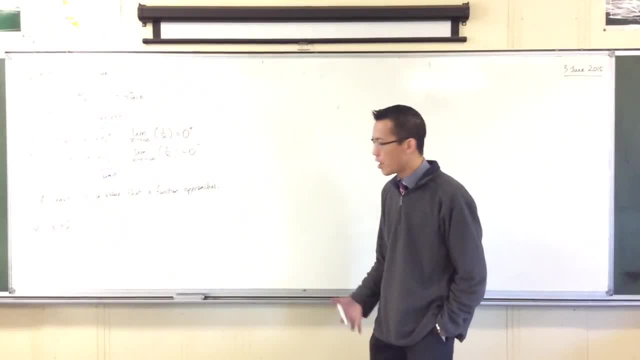 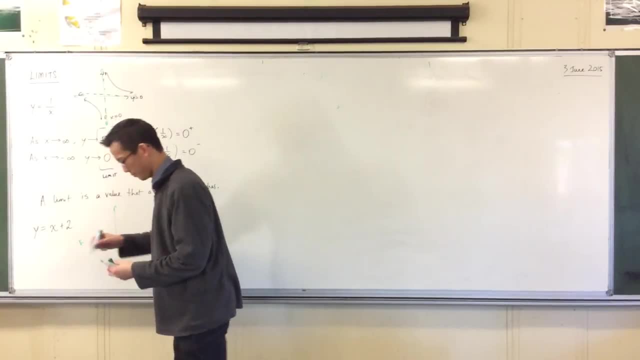 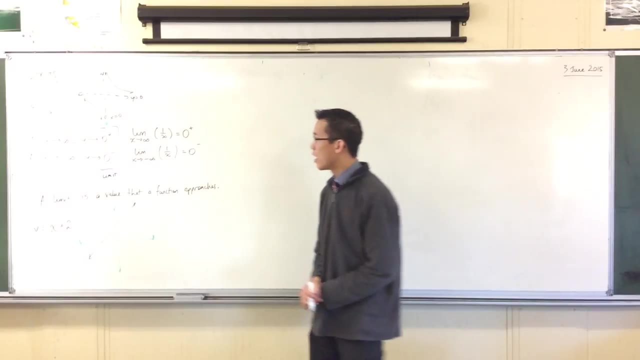 y equals x plus 2.. Okay, Now I can graph this. I can graph this. It's not a hard thing to graph. There's my: y equals x plus 2.. Okay, Now x can approach infinity and x can approach negative infinity. 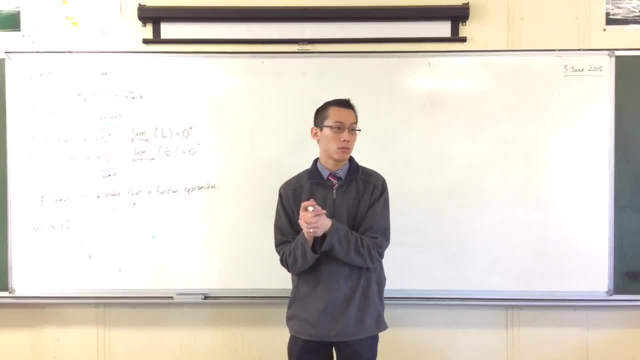 The only reason why I choose those values is because that will give me a horizontal asymptote. But I can approach any value I like And I can see what happens to this guy as I approach that value. So, for instance, I can think about the limit as x approaches, say, 0.. 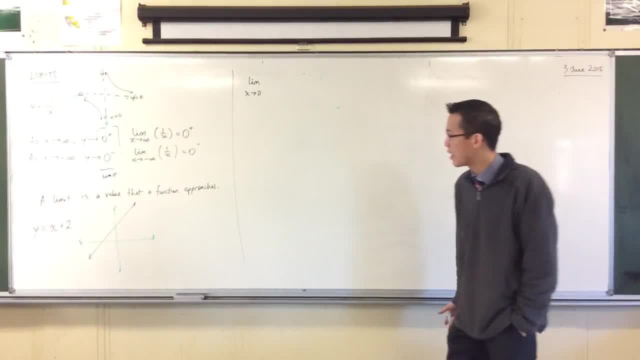 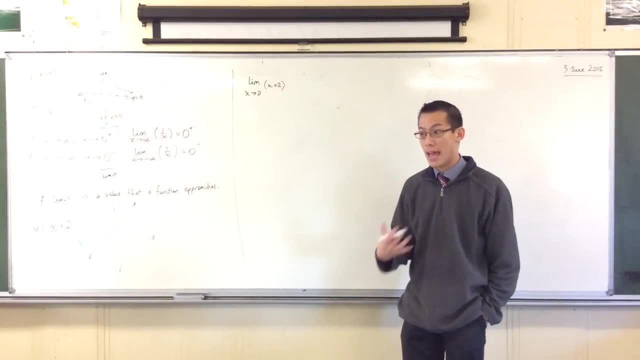 There's a number. I can go ahead and approach that and see what happens. Right, What happens to x plus 2 as x gets smaller and smaller and smaller? Okay, And the answer is: well, let's just think about it this way. 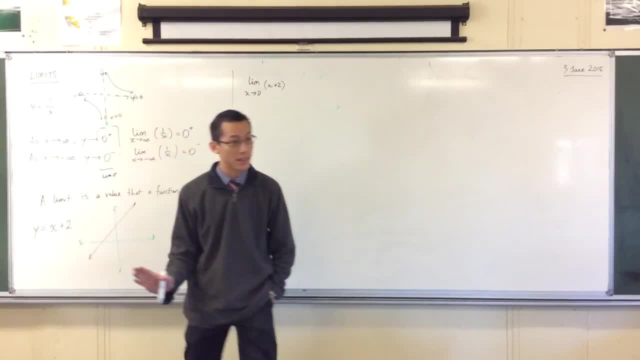 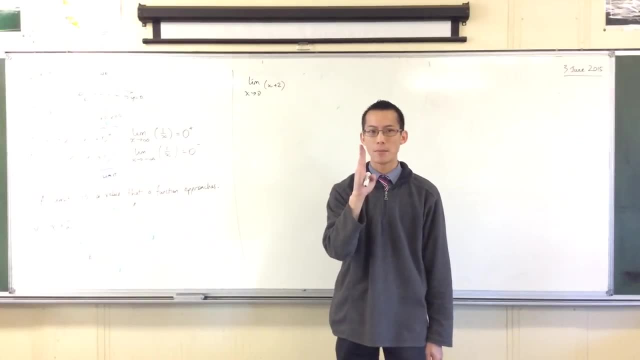 I can approach. there's x equals 0 on the y axis, Right. Unlike positive and negative infinity, I can approach 0,. I can approach it from two angles, Can't I Right? I can come from the right or I can come from the left. 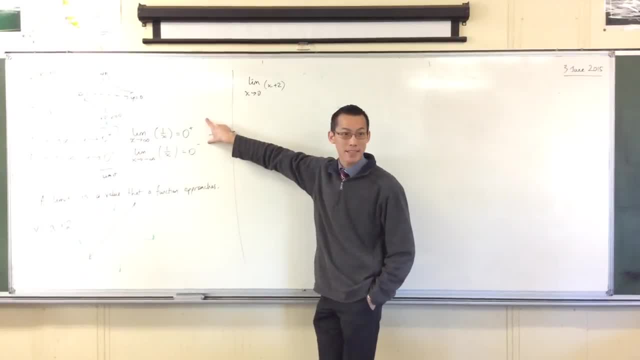 Okay Now, thankfully, we have already developed language to talk about that, Right From above or from below. So what I can say is: well, let's think about coming from the right-hand side, From 0 but above. 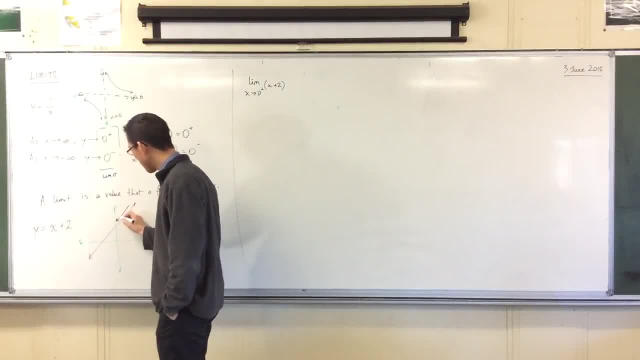 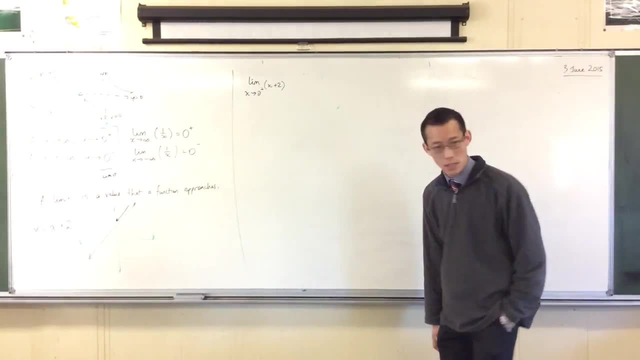 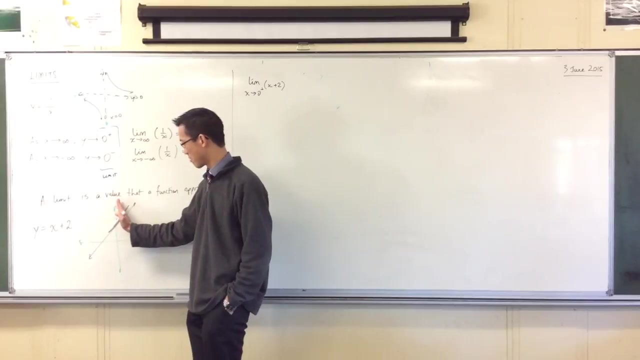 Okay, So here's where I'm going. That's the direction I'm going in From above, and I'm going towards 0.. Okay, So what's going to happen to x plus 2?? As I'm getting closer and closer to x equals 0, right y is getting closer and closer to 2.. 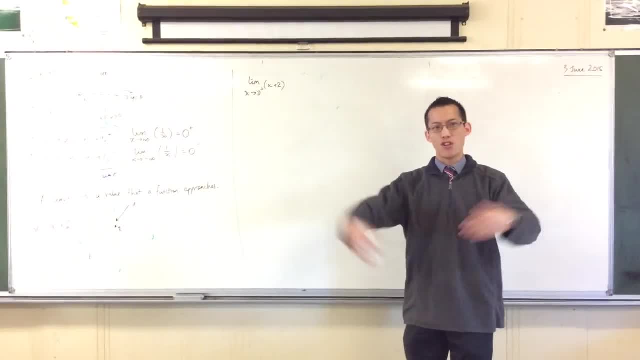 Okay, Closer and closer and closer. In this case, there are no discontinuities, There are no asymptotes. We can actually get to 2.. Okay, So there's no problems. I can still this idea of the limit right, we first meet it with regard to asymptotes. 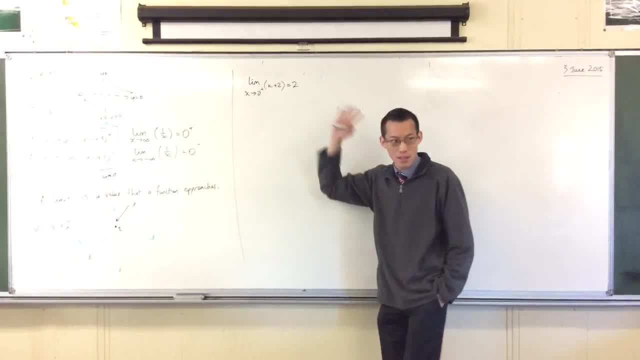 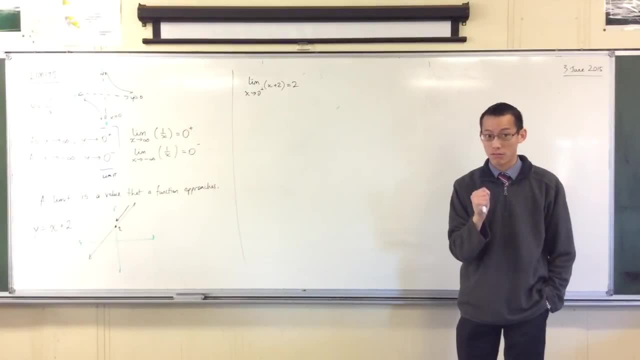 because that's where it's relevant. But you don't have to have asymptotes to think about limits. It's just what a function approaches, Okay. So, yes, you should. Yes, you should. Now. here's the thing, though. 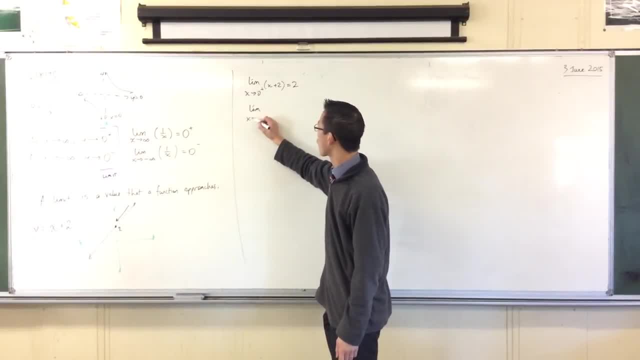 You will notice, right, if I now think from the other side, from below 0, so that's coming from this direction. okay, you can see that if I put in like what's happening to this, I'm still approaching the same number. 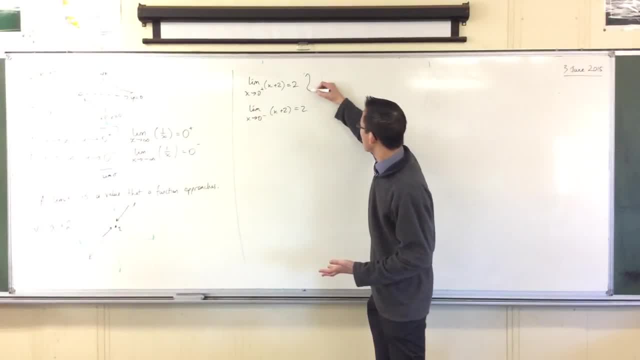 I'm still approaching the same number. So in some ways I can combine these two right, because wherever you approach 0 from right, as x approaches 0, you can come from above, you can come from below- it's still going to go toward 2.. 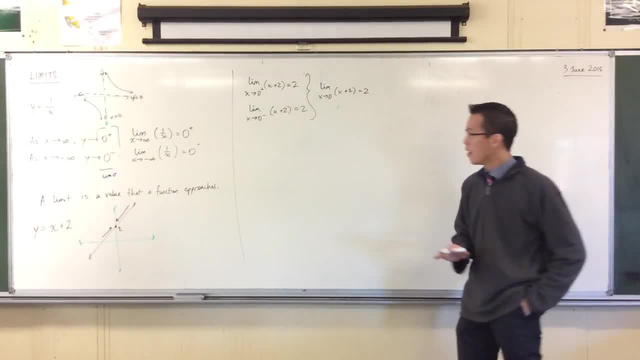 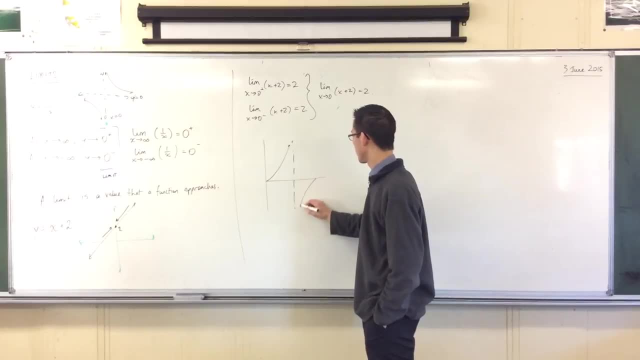 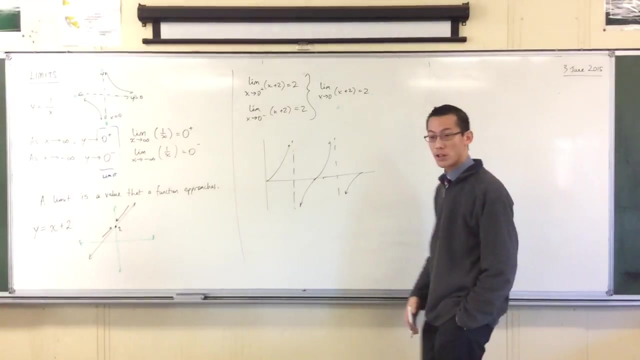 Okay. Now, this is not always the case. This is not always the case. For instance, let's think about this guy. This graph, of course, is tan x Okay. So if we just do regular old tan x okay because of all these asymptotes flying around, right? 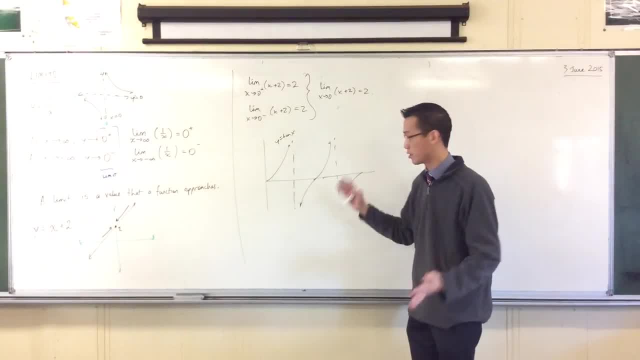 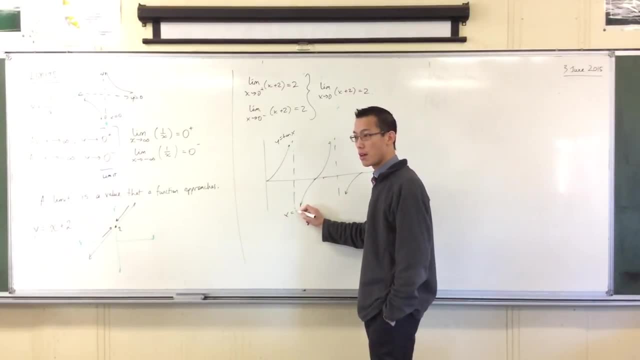 and all of these parts where there are breaks in the function. okay, I have an asymptote. well, actually I have two asymptotes here, and their equations are: x equals 0.. Okay, And their equations are: x equals 90 degrees and x equals 270 degrees. 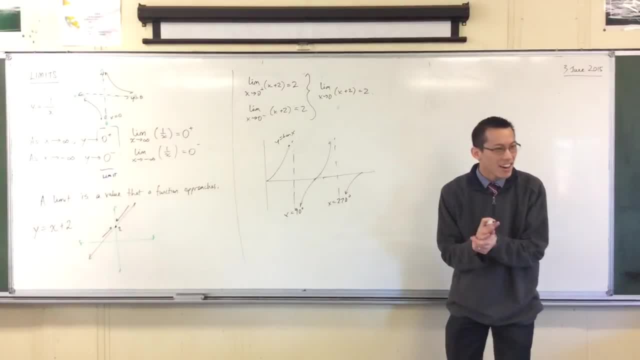 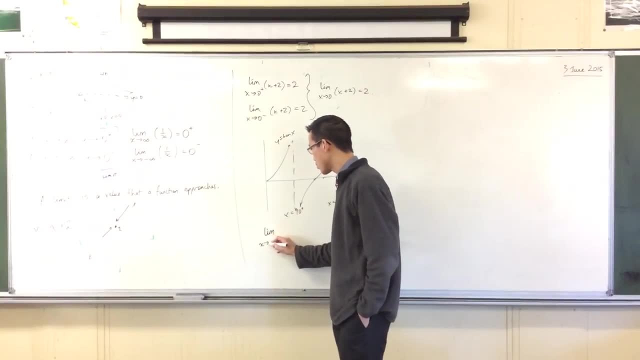 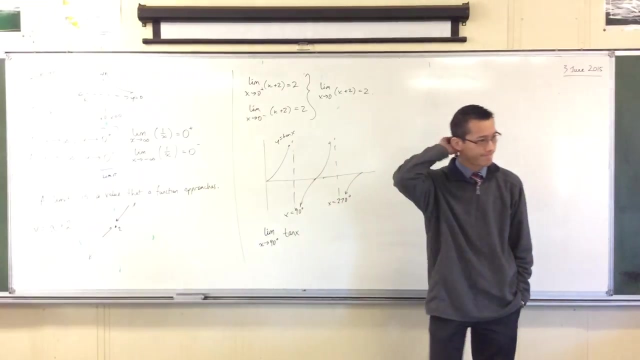 Okay, That's what I meant to say. Okay. So now, for instance, in this case, let's think about what happens when we think of the limit as x approaches one of these asymptotes right of this function. Hmm, 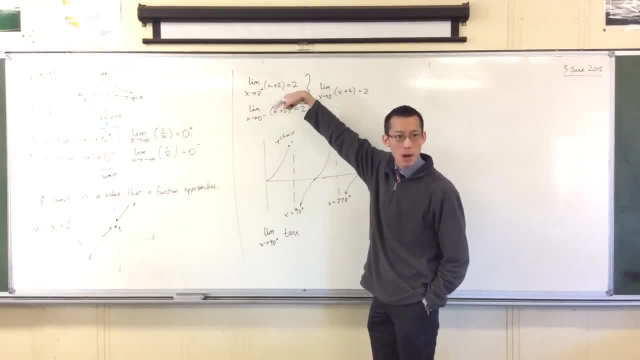 Okay, So here this whole- which way do you come from? this kind of makes a big deal, doesn't it Right, Like if, for instance, I come from the right-hand side? okay, from above 90 degrees. 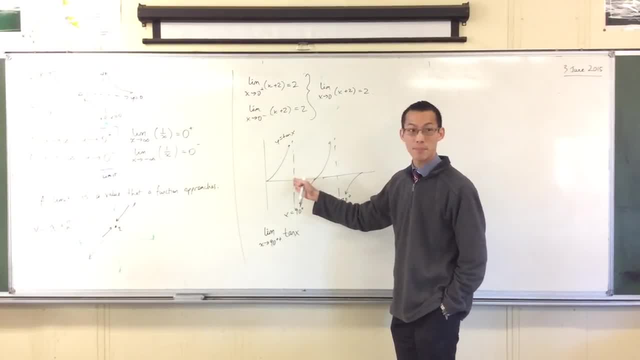 So here's like 91 degrees and 90.5 degrees and 90.05 degrees, and on and on and on. Okay, What am I approaching as I get closer and closer? What does tan x approach? 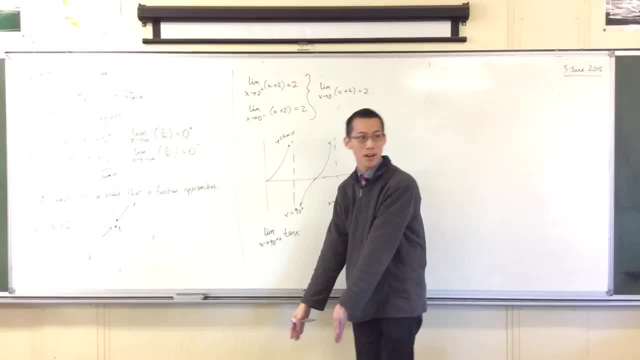 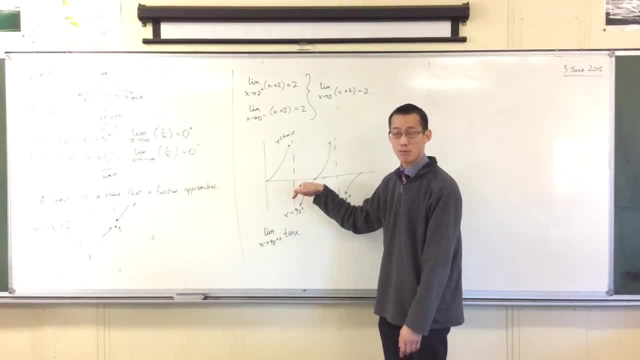 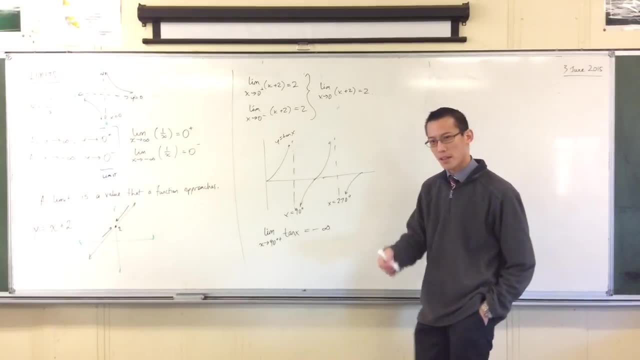 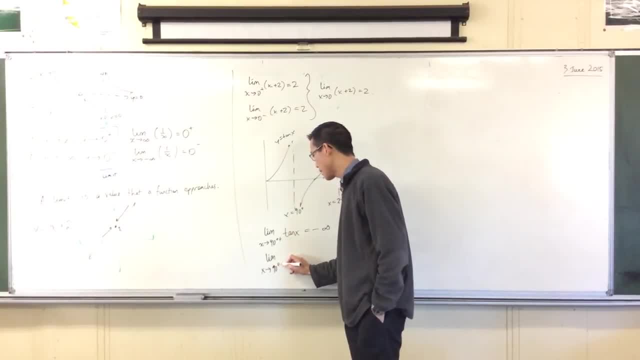 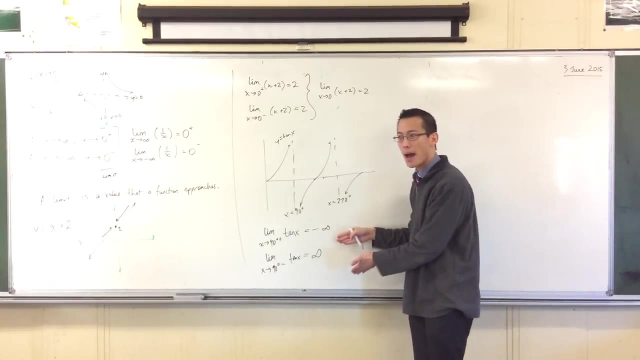 go towards the left right. if I go from the other side, right from below, okay, tan x is not going to negative infinity, It is going towards infinity. Okay, Whoosh Off it goes. Okay. So this guy, I cannot combine in the way that this guy does, right. 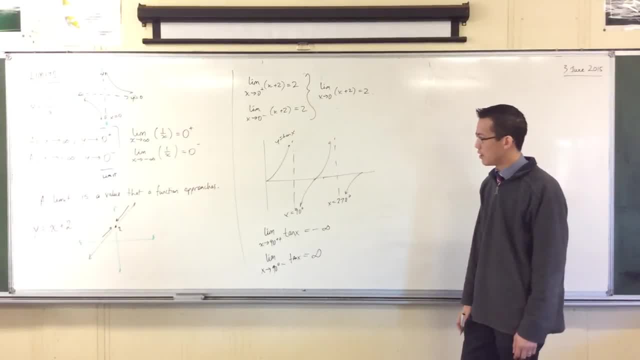 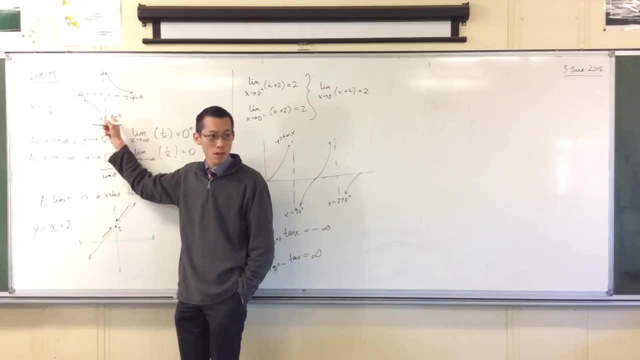 Because if I just say, if I just say, as x approaches 90, is it positive or negative infinity? Well, that kind of makes a difference, doesn't it right? It's exactly the same over here. As x approaches zero, right, like? well, which side do you want to come from? 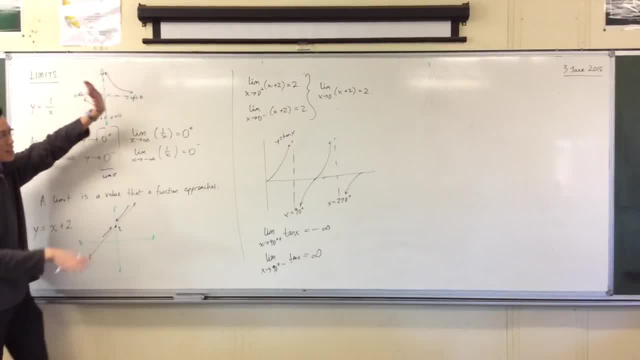 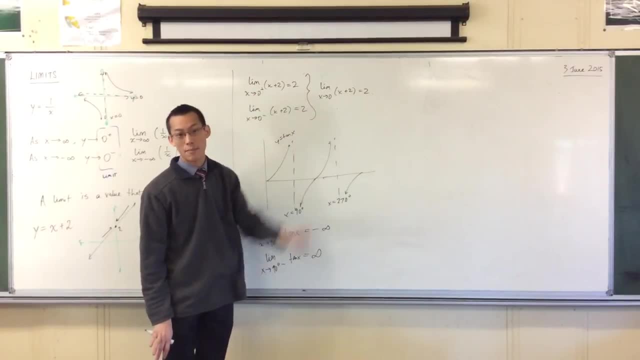 Because you will get opposite things Okay. So this idea of the limit right the side that you come from matters, but sometimes, whichever side you come from, you'll get the same thing, Okay. So you will often, depending on the functions you get, you will often get no sign on this. telling you which way to come from.